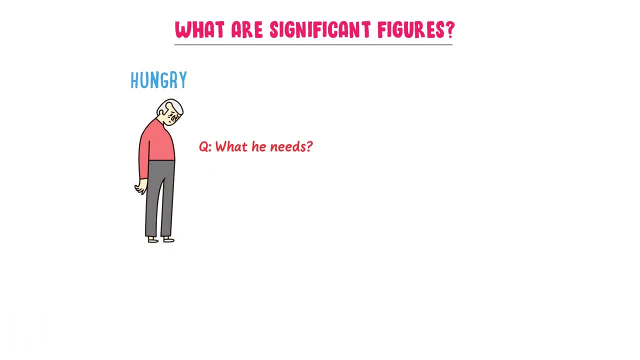 Let me ask you what he needs in order to kill his hunger. Well, the answer is simple: He needs food in order to kill his hunger. Here we say that food is important. Secondly, it is certain that food will relieve his hunger. 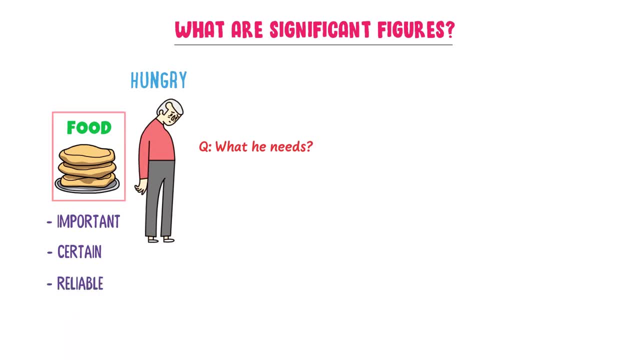 Thirdly, we say that food is a reliable source. Also, consider that this hungry man adds some fruits to his food. Let me ask you: is it important to add fruit to his food? Well, your answer is: it is not that much important. 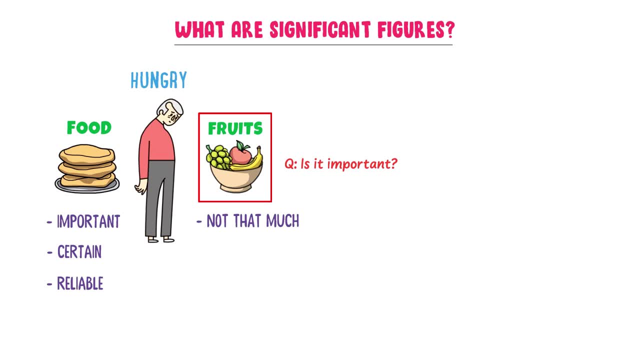 because hungry man can kill his hunger only by the food. But remember that we cannot ignore its importance. Similarly, consider a table Let. the length of this table is 122.3 cm. Now I take the first three digit: 122.. 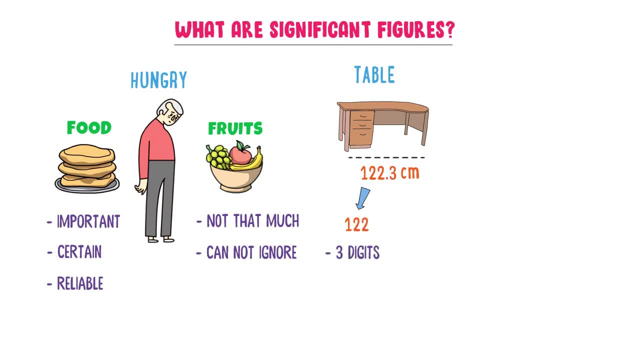 We know that this is a three digits number. Secondly, we are certain about them. For example, the length of the table is 122 cm. Also, we say that it is a reliable number. Personally, I call this number as a two digits number. 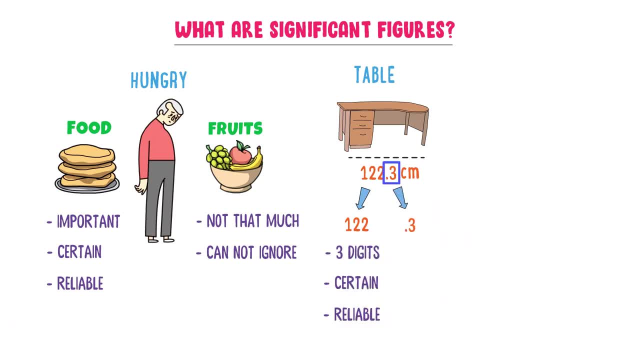 On the other hand, I take the decimal part, 0.3.. We know that it is one digit number. Secondly, we say that it is uncertain. I mean it is not uncertain, It is not that much important to be included. 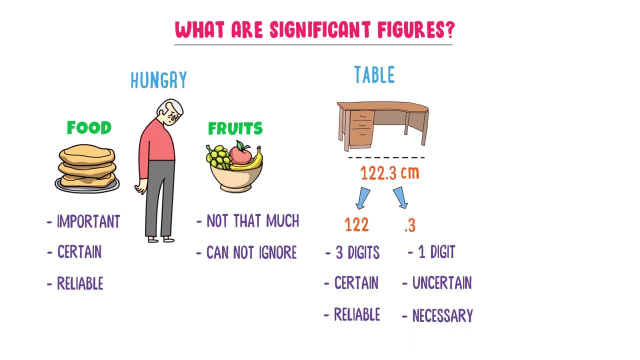 But it is necessary, like fruits, to be indicated. Thus we say that there are four important digits present in this measurement, Or we say that there are four significant figures present in this measurement. Therefore, we define significant figures as the certain and necessary digits in any measurements. 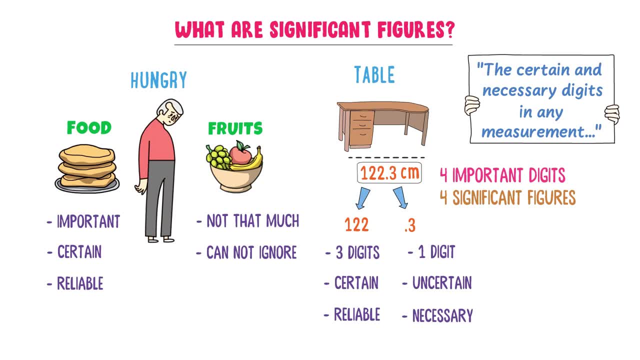 are called significant figures. Let me repeat it: The certain and necessary digits in any measurements are called significant figures. For example, in the 122.3 cm, there are four significant figures. Thus note it down, this easy definition of significant figures. 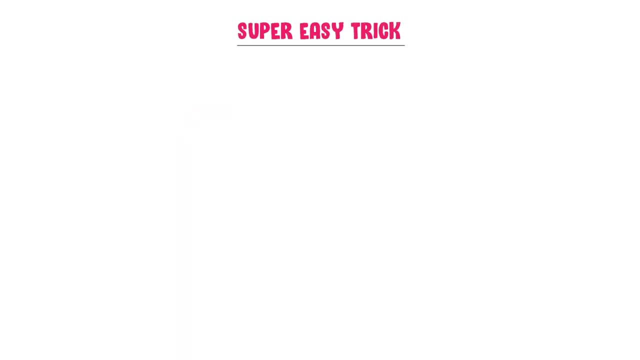 Now let me teach you the super easy trick in order to identify the total number of significant figures in any number. We know that We have two types of numbers, like non-decimal numbers and decimal numbers. In case of non-decimal numbers, the trick is go from first non-zero digit to the last. 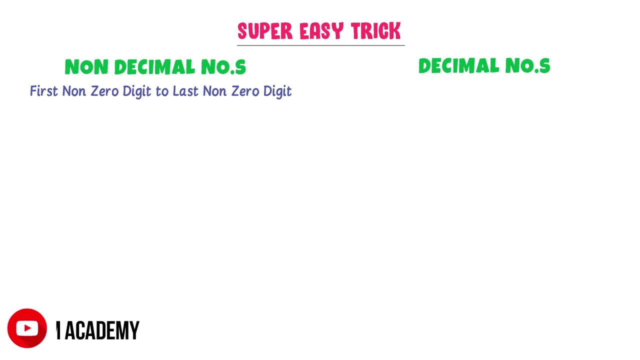 non-zero digit. Let me repeat it: Go from the first non-zero digit to the last non-zero digit. For example, consider this number. We know that one is a non-zero digit number. Now the last number, six, is also a non-digit number. 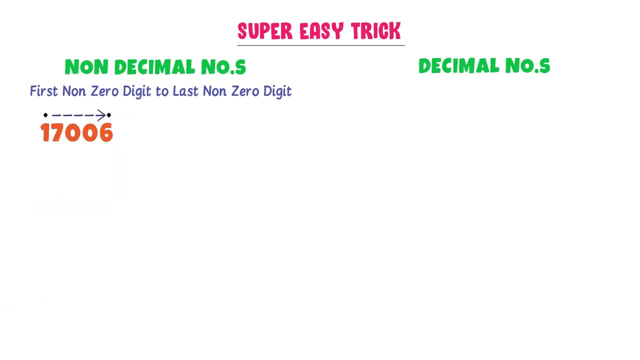 So I will go from one to the six. Now, one, two, three, four, five. So we say that there are five significant figures present in this number. Secondly, consider this number. We know that the first digit is one and the last non-zero digit is seven. 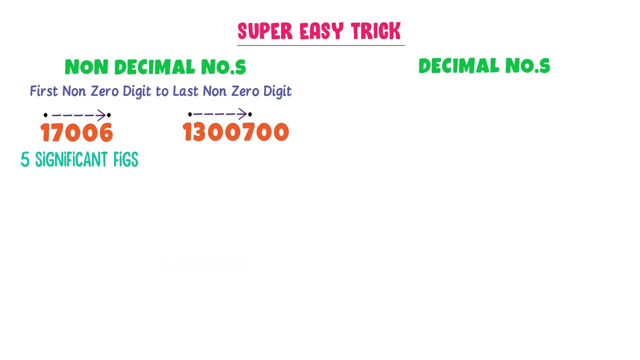 So go from one to seven: one, two, three, four, five. There are five significant figures present in this number. Thirdly, consider this number: The first digit is four and the last non-zero digit is also four. So I go from this four to this four: one, two, three. 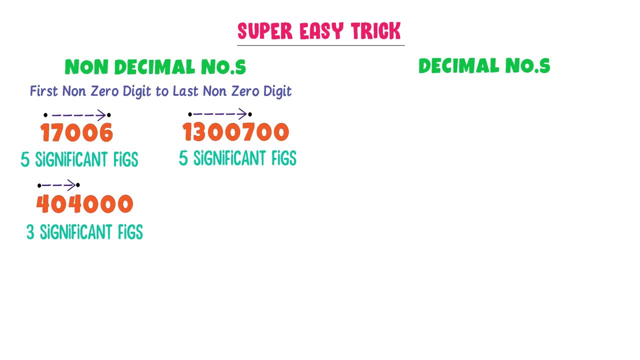 There are three significant figures present in this number: Four, three, four, five. Fourthly, consider this number. The first non-zero digit is five and the last non-zero digit is two. So go from five to two. one, two, three, four, five. 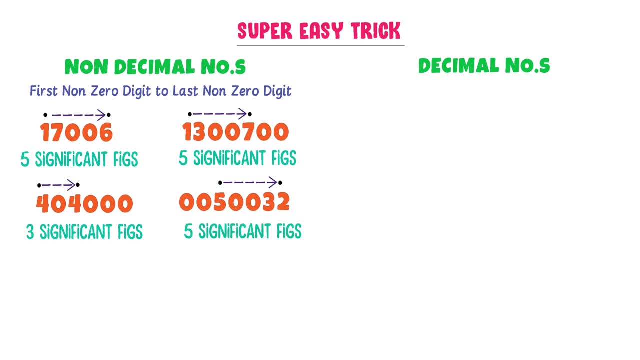 There are five significant figures present in this number. Fifthly, consider this number: The first non-zero digit is six and the last non-zero digit is one. So I go from six to the one: One, two, three, four, five, six, seven. 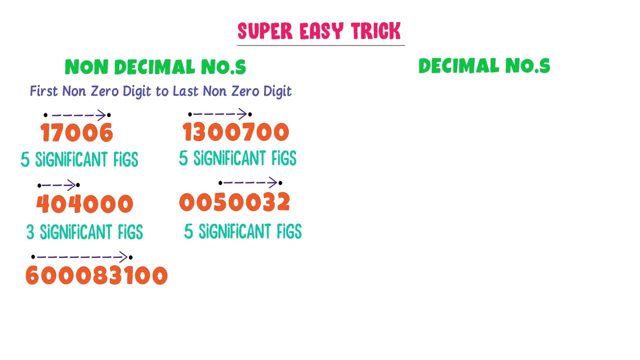 There are seven significant figures present in this number. Finally, consider this number: The first non-zero digit is nine and the last non-zero digit is three. So go from nine to three. one, two, three, four, five, six. 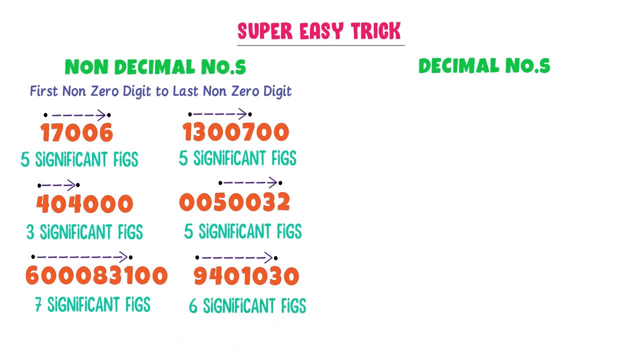 So there are six significant figures present in this number. Six, Three and this number. Thus, by this way, we can easily find significant figures in any number. Now, in case of decimal numbers, go from first non-zero digit, Let me repeat it, Go from: 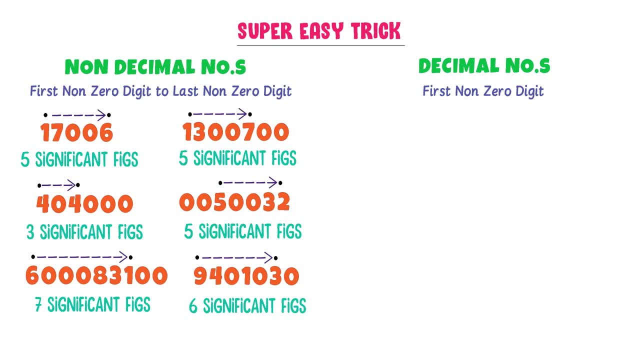 first non-zero digit And it is always the difficult part for the student, But I will make it super easy for you. For example, consider this number: The first non-zero digit is 2.. So go from the 2 to the last: 1,, 2,, 3.. So there are 3 significant figures in. 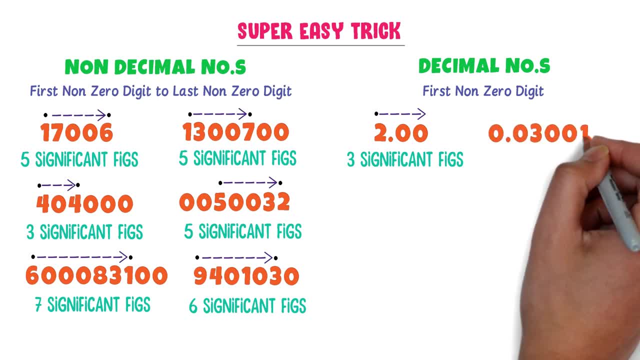 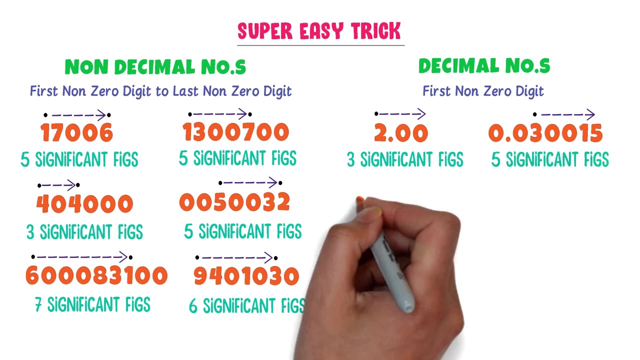 this number. Secondly, consider this number. We know that 3 is a non-zero digit, So go from 3.. 1, 2, 3, 4, 5.. So there are 5 significant figures present in this number. Thirdly, 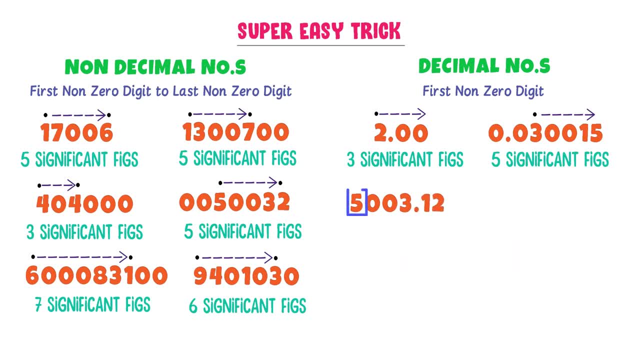 consider this number, We know that the first non-zero digit is a non-zero digit, So go from 5.. 1, 2, 3, 4, 5, 6.. There are 6 significant figures present in this number. Fourthly, 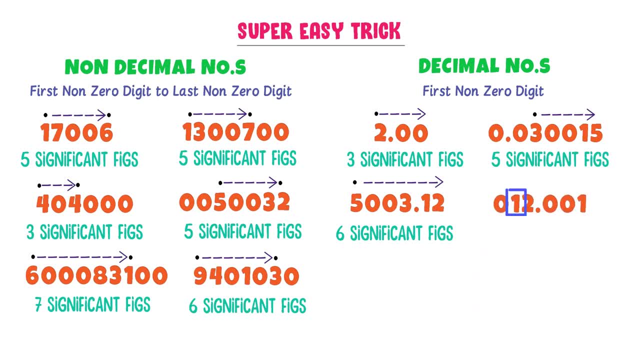 consider this number. We know that the first non-zero digit is 1.. So go from 1.. 1, 2,, 3,, 4, 5.. There are 5 significant figures present in this number. Fifthly, consider this number. 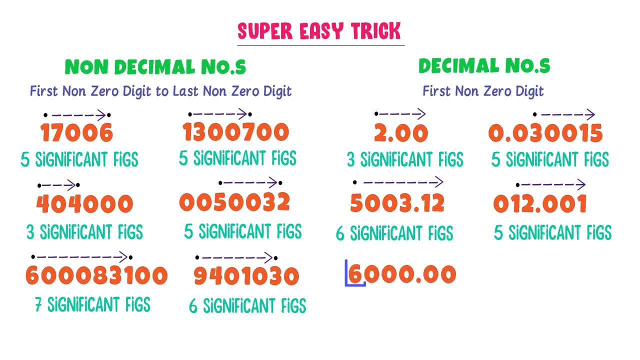 We know that the first non-zero digit is 6.. So go from 6.. 1,, 2,, 3,, 4,, 5,, 6.. There are 6 significant figures present in this number. Fifthly, consider this number The first non-zero. 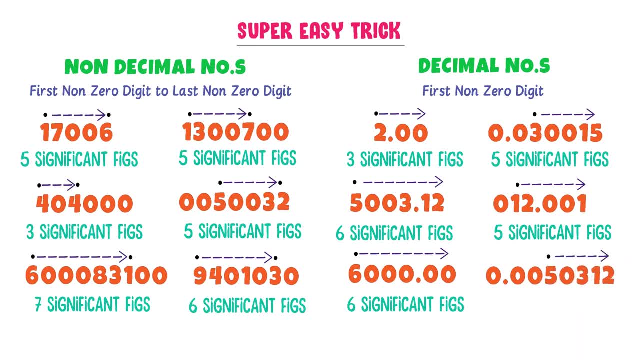 digit is 5.. So go from 5.. 1,, 2,, 3,, 4,, 5.. There are 5 significant figures present in this number. Thus, by this way, we can easily find the significant figures in any number.